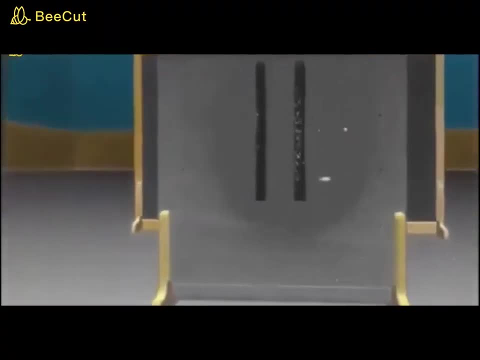 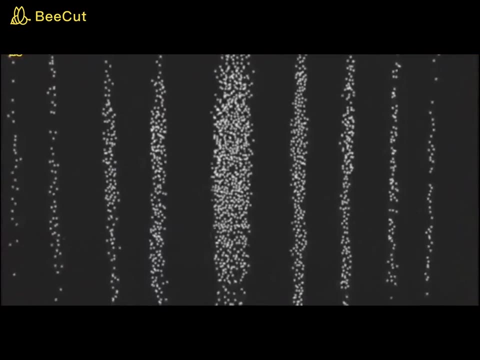 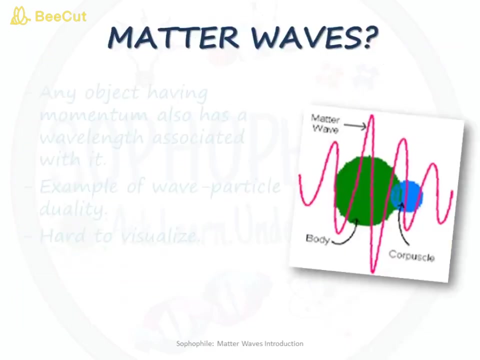 We can see this wave behavior of electrons by Davis and Gutterman experiment. It is observed that each electron is detected at specific place and time like a particle, But on repetition of experiments many times we can see a pattern of stripes characteristic of wave behavior. Understanding what is a wave and particle, then, what are matter? 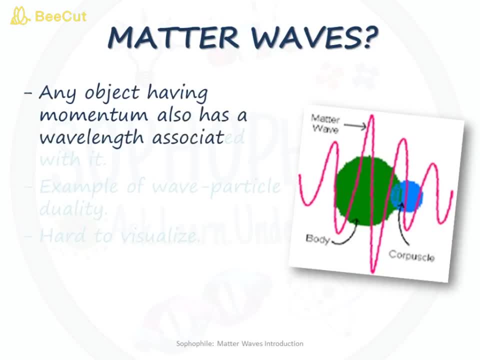 waves. Any object is a wave and particle is a particle. Then what are matter waves? Any object having momentum also has a wavelength associated using matter and earth. Matter wave is an example of duality of wave and particle. Matter waves are hard to visualize since we consider matter as 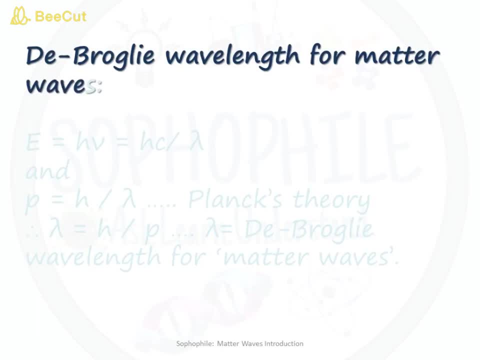 solid instead ofLING tIn one's Morocco saviour. The wave length associated with matter waves is a matter waves. Energy is equal to h, nu, which is equal to hc by lambda, And in Planck's theory, lambda is equal to h by p. 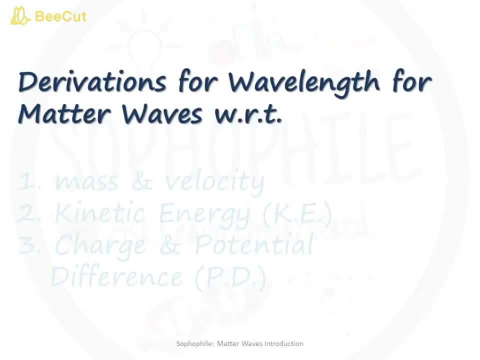 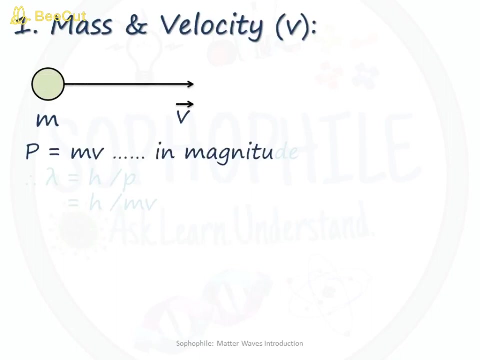 ți is the wavelength between the matter waves and h is the Planck constant for wavelength for matter waves, with respect to: first, mass and velocity. second, kinetic energy. third, charge and potential difference. first, mass and velocity. consider a particle with mass m and velocity v moving in a certain direction. therefore, its momentum is. p is equal to mv substituting p. 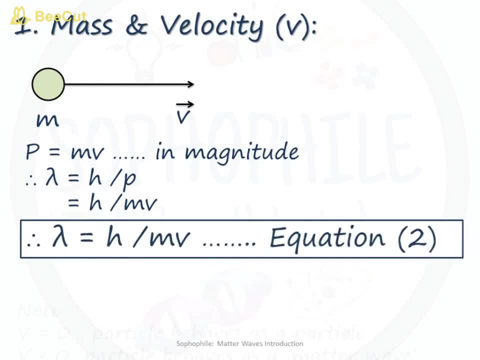 is equal to mv, we get lambda is equal to h by mv. it is important to note that velocity is zero, then particle behaves as a particle and when velocity not equal to zero particle behaves as matter wave. de broglie wavelength of matter waves with respect to kinetic energy. we know that kinetic energy is: 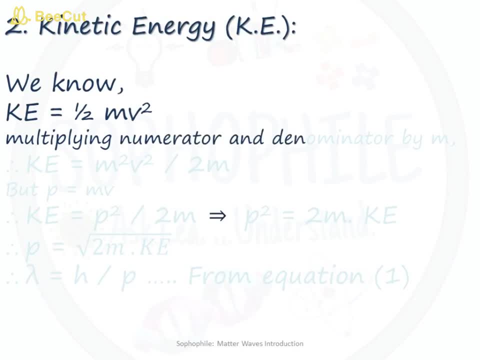 equal to one half mv square. therefore, kinetic energy is equal to m square v square by 2m. therefore, ke is equal to p square by 2m, which implies p square is equal to 2mke. taking under root p is equal to under root of 2mke. therefore, substituting this: 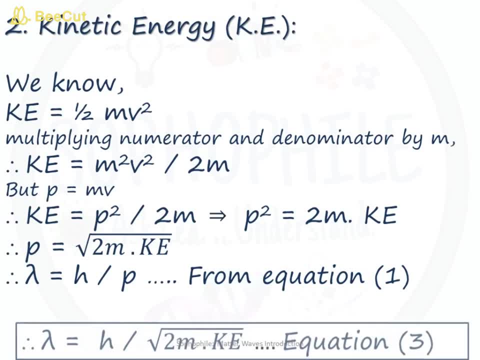 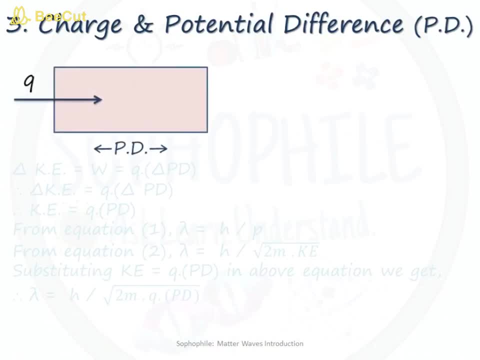 in first equation we get de broglie. wavelength is equal to h upon under root of 2mke. third, charge and potential difference. consider a conductor with charge q and potential difference pd. then change in kinetic energy is equal to work done, which equals to charge into change in pd.